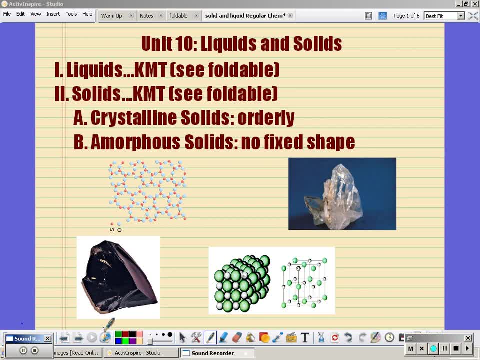 This is Unit 8, liquids and solids. The kinetic molecular theory of liquids and the kinetic molecular theory of solids are in the foldable. Make sure that you complete the foldable and look at the properties discussed on the foldable and know the differences between those properties. 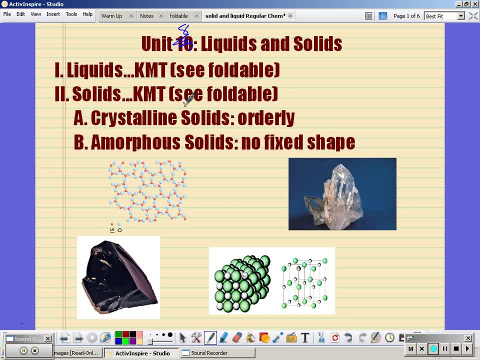 in reference to solids, liquids and gases, You're going to have to remember some things from Unit 7.. There's two types of solids. There are crystalline solids, which are very ordered, and there are amorphous solids, which actually have no fixed shape. So, if we look, 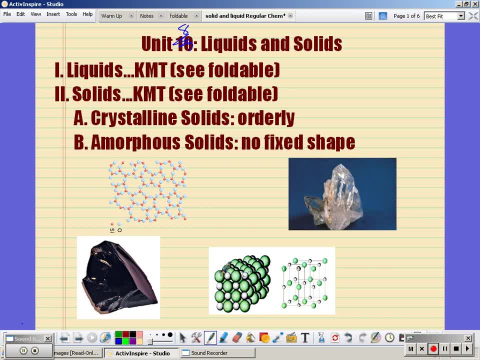 at our pictures down here at the bottom we have sodium chloride. So you have chlorine sodium, chlorine sodium, chlorine sodium. It's a very structured. there's a pattern to it. So that is a crystalline structure. An amorphous solid is like the SiO2 here. 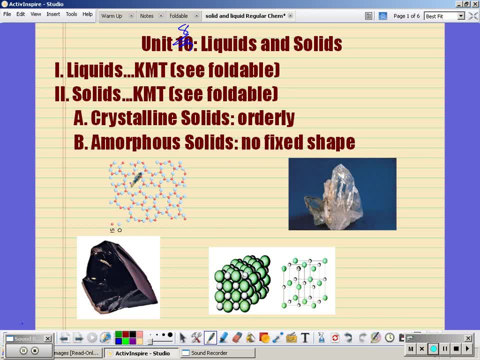 We don't have a specific structure. None of the circles are identical, So there's no fixed shape, so it's an amorphous solid. There are two amorphous solids that you need to be aware of, and those are our plastics. 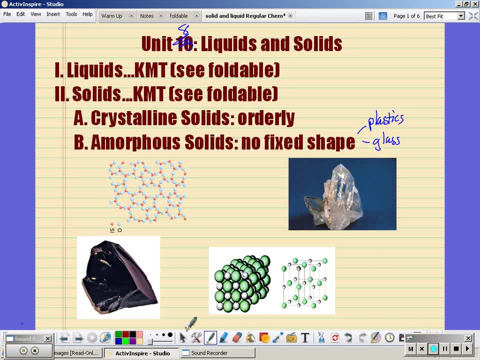 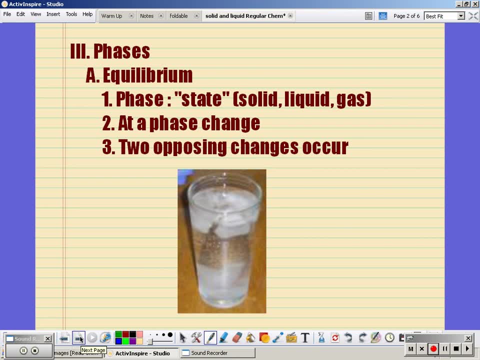 and glass. Both plastic and glass are amorphous solids, Phases. Phases exist in equilibrium, In other words, we have two phase changes occurring at the same time and they're opposites of each other. So in my glass of water, 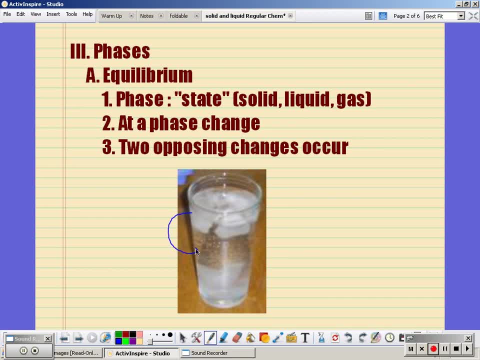 I have ice turning into liquid water, So I have solid going to liquid and we call that melting. But at the same time some of my liquid hits the cold ice cubes and goes back from liquid to solid, which we call freezing. So I have the two opposing changes melting. 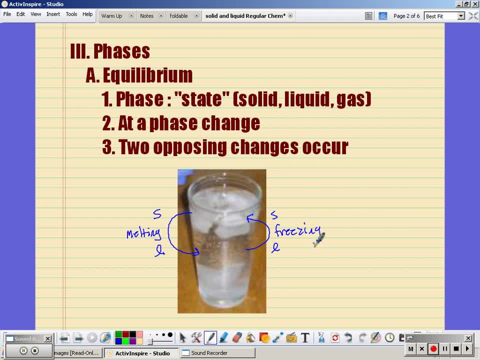 and freezing occurring at the same time. So my glass of water is at zero degrees Celsius until everything turns to a liquid or everything turns to a solid. then the temperature can change. So, equilibrium: we have these two opposing phase changes occurring and the temperature. 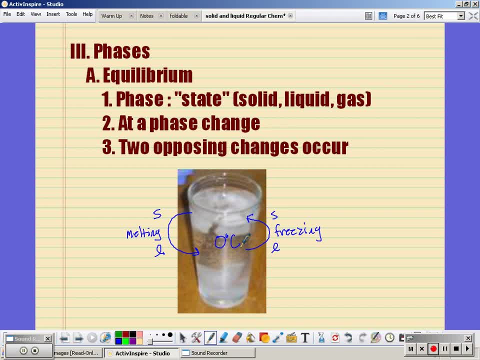 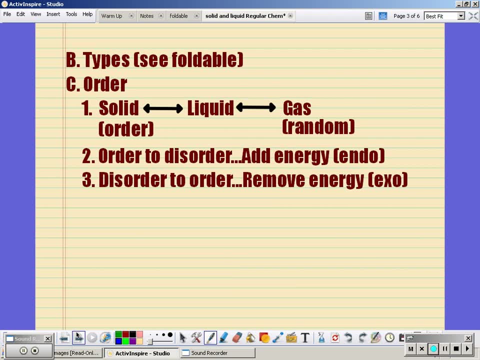 remains constant until everything changes to one phase. So all of our phase changes happen in these pairs. As you go from something very ordered to something very random, or you'd go from random to very ordered, you have a change in energy. If you have to add energy in, then it's endothermic. 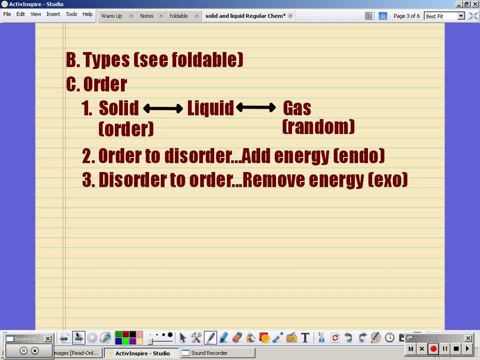 If energy is removed, it's exothermic. We've known those two vocab words since Unit 1.. If you are creating disorder, if it's becoming disordered, then it's endothermic. So as we move from solid to liquid to gas, it is an endothermic process As you become more ordered. 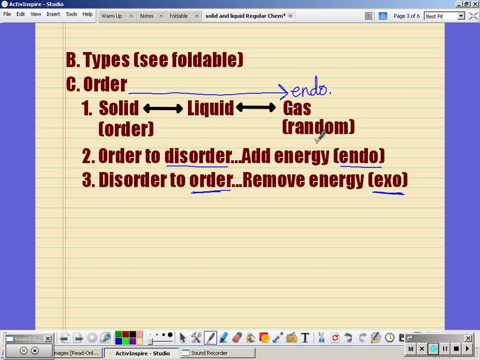 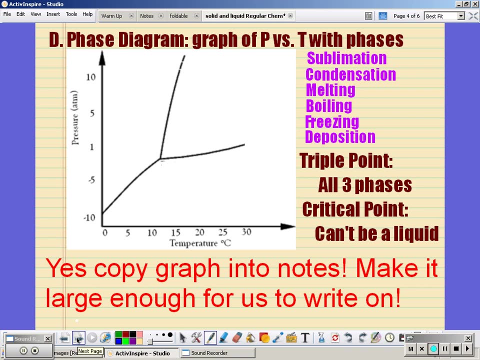 or less random, then it's an exothermic process. So as you go gas to liquid to solid, it is exothermic. Now a phase diagram represents the pressure and temperatures of our different phases and how we can change pressure and temperature to create our phase changes. So the area that's next to the x-axis is always our solid area. 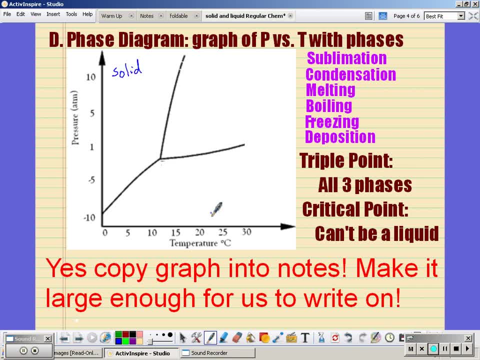 The Benjamin Jakob Larkin, 06 vào James H cataler 06 vao. next to our y-axis is always our gas area and the area that's in between is always our liquid area. so if we were to move across the line from liquid to 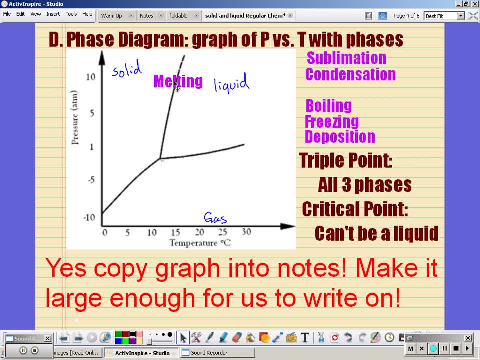 solid, we would call that melting. so if we were to start in this area and end in this area, the line would tell us the melting point. if we were to start in the liquid area and go to the solid area, that would be called freezing. so moving from this side to this side of the line is freezing. so the freezing point would 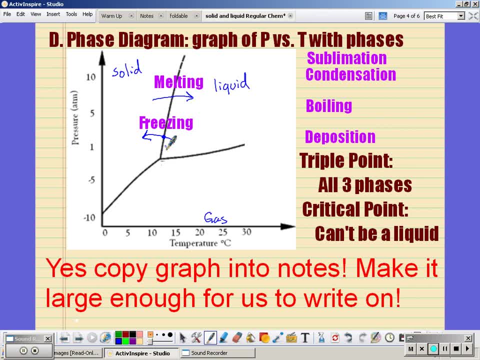 occur on that line now. if we were to go from the liquid to the gas phase, that would be called boiling. if we were to move from the gas to the liquid phase, that would be called condensation. so it depends which direction or how you're moving across the line, to what 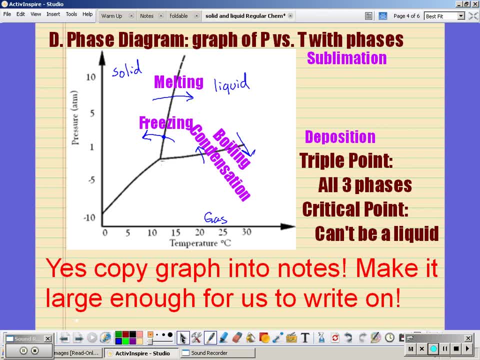 vocabulary word you're using. if we go from a solid to a gas, that's called sublimation, so we'd have to be crossing the line that direction. the opposite would be deposition: going from a gas to a solid, so we would be crossing the line that direction. 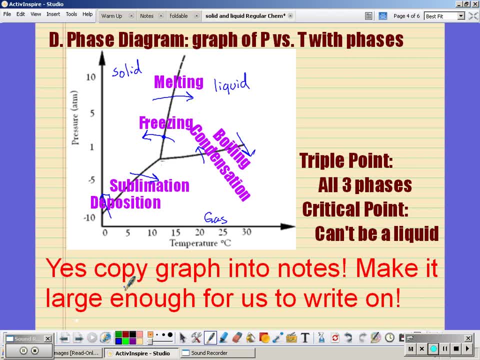 now the triple point is where all three phases coexist together. so right here, where our three lines meet, that is the triple phase or, I'm sorry, the triple point. so at that temperature, at that pressure, you would see the solid, the liquid and the gas of that substance. 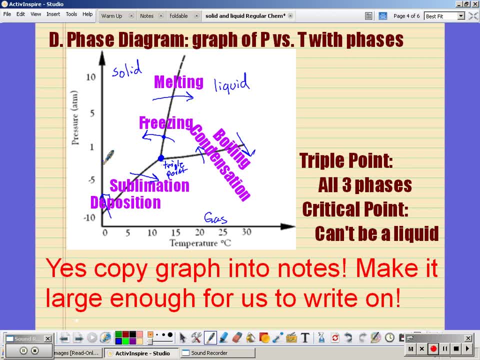 together. the critical point is where you can no longer be a liquid, so that's the point where the liquid to gas line ends. so you'll be asked questions like: at 5 ATM and 5 degrees Celsius, what phase are you? and so you could say, well, at 5 ATM and 5 degrees Celsius, I'm a solid if I 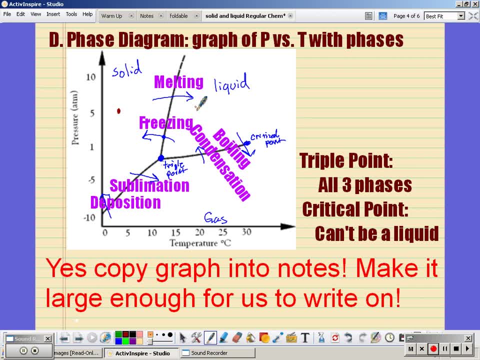 was to increase the temperature to 20 degrees Celsius, what phase change would occur? I would say melting, because I'm going across the liquid solid liquid phase, the line, that direction. another question is: what is the normal melting point? well, normal means 1 ATM. melting means going from solid to liquid. so if I was at 1 ATM I'd come across and I would come down and I would mark down my temperature. so let's say it's 11 degrees Celsius, because it's pretty close to 10. so the melting point would be 11 degrees Celsius, the normal melting point 11. 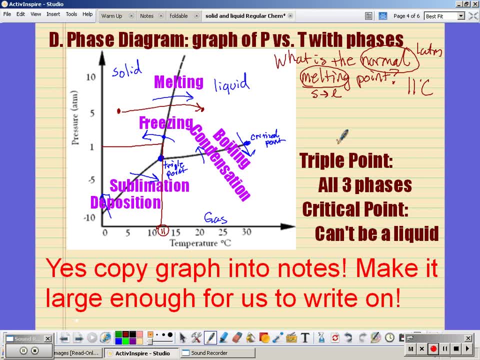 degrees Celsius. if it said what is the normal boiling point, I know normal means 1 ATM and I know boiling means liquid to gas. so I would just continue my line over till I hit the liquid to gas line and I'd come down and that looks about. 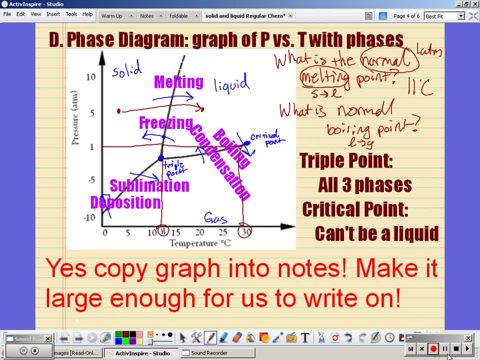 to be 30 degrees Celsius. what is the normal melting point? the normal melting point is my 1 ATM one day upgrade. how much heat do I need to vaporize liquid from 1 ATM one day? for example, if I'm going to vaporize or I'm going to heat my liquid up, I need